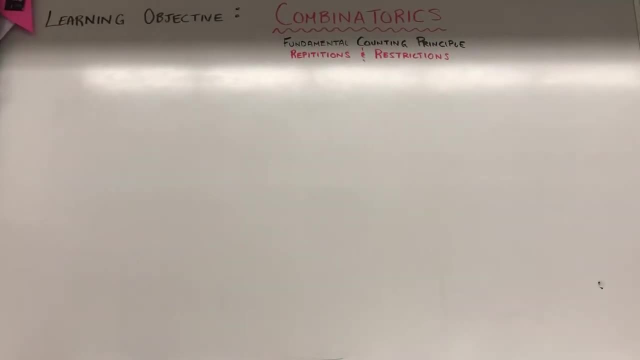 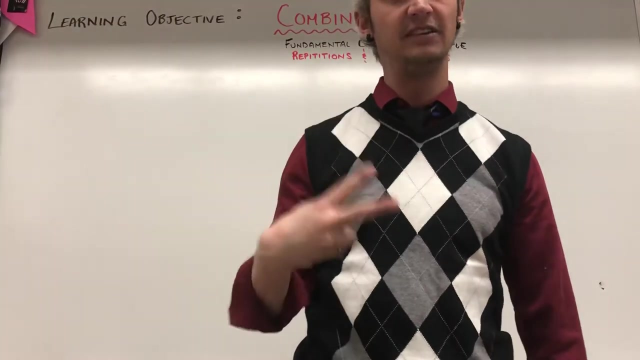 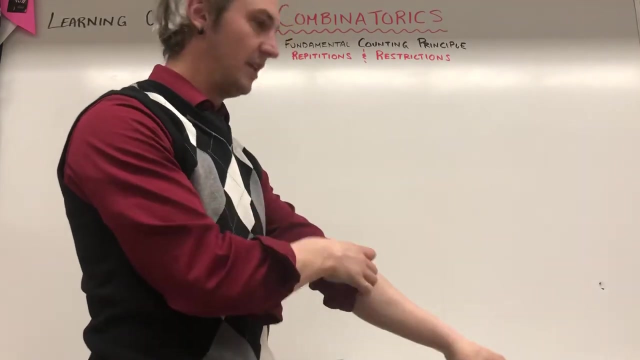 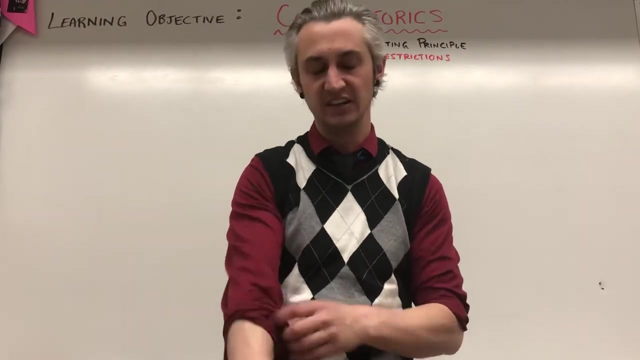 Oh, oh, yeah, cool. Okay, what is happening, my little babies from the 403 to the HAZ? Mr Nelson, here We are talking about combinatorics and combinatorics is just an investigation of the different ways we can arrange objects, ideas, objects, ideas, same thing. And in the last video, kind of our introductory video, we talked about the 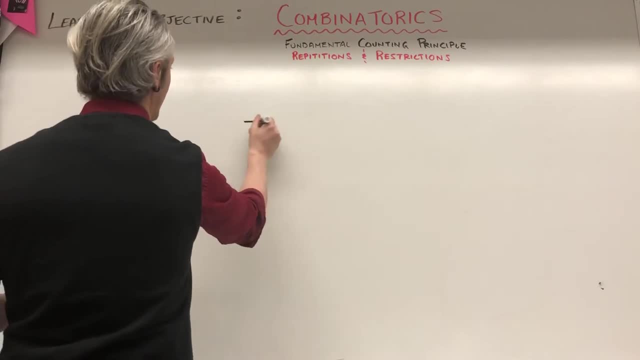 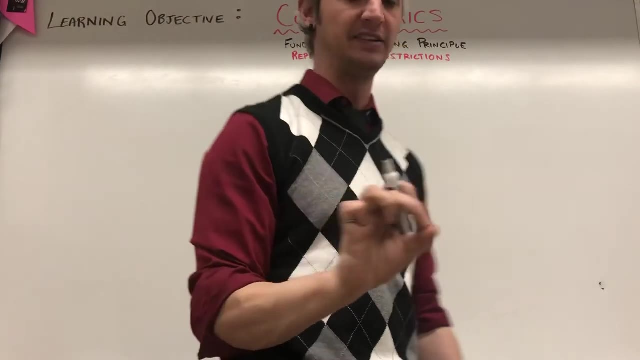 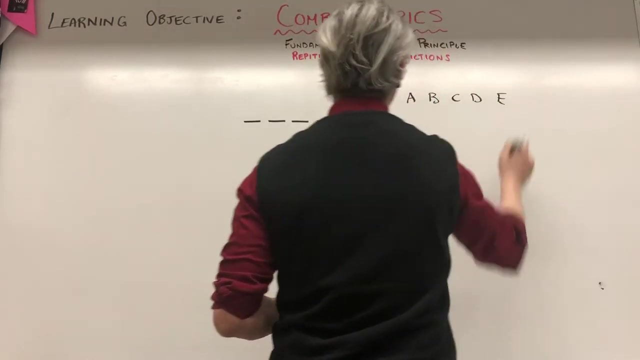 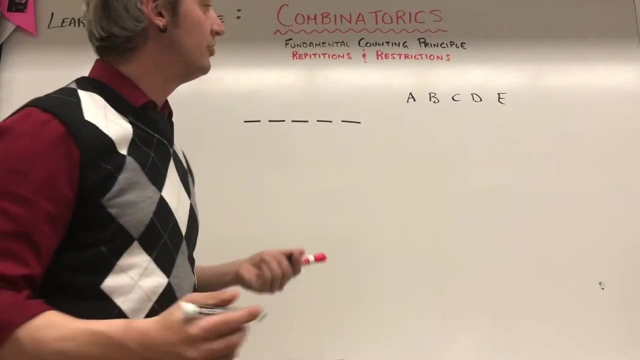 notion of factorial, right? So when I'm trying to arrange five objects, see all the different ways I can. I can arrange five different objects, right, So there's no repeats. So, like you know, ABCD, ABCDE, Okay, right, figuring out how, all the ways I can arrange these is basically just taking the amount of unique objects and doing factorial. So I have five objects. I'm trying to figure out how many ways I can arrange them. I can do that five different ways. 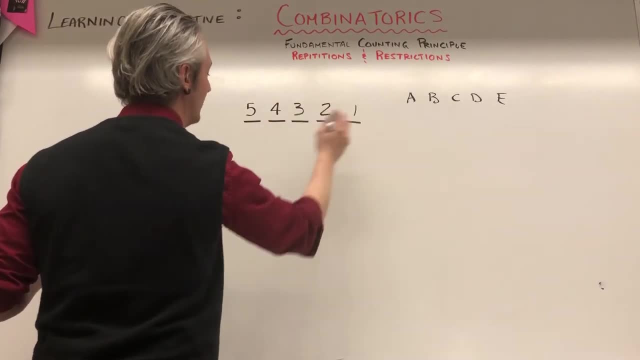 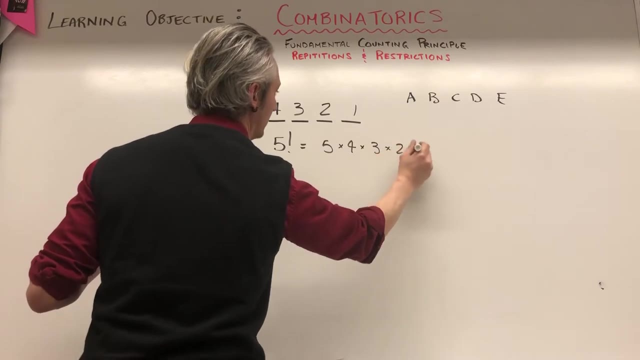 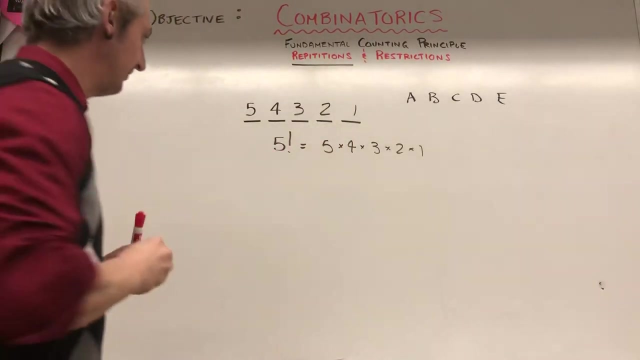 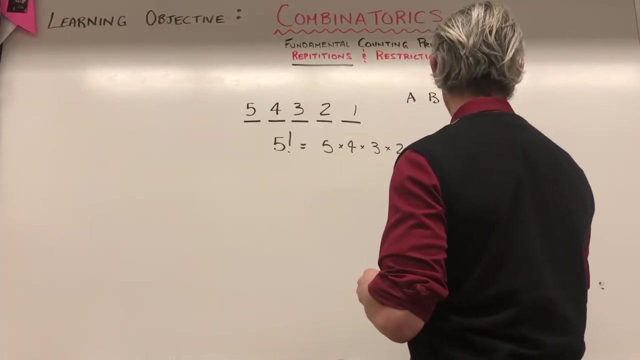 This one. I have four to choose from. three left to choose from two left to choose one. five factorial equals five times four times three times two times one. Now, the first thing we're gonna look at is what happens when we have repetitions. okay, So what would happen if, instead of ABCDE, I had ABCCD And I said: how many unique? unique, whereas C is the same as C. 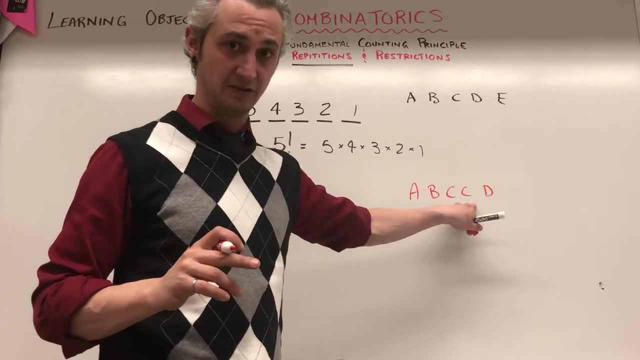 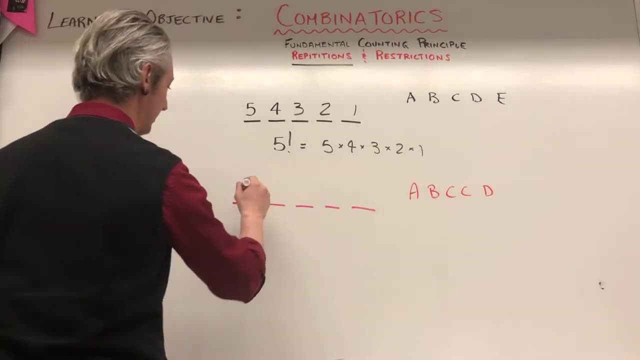 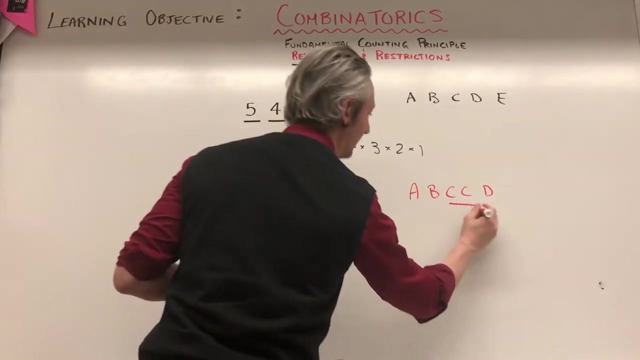 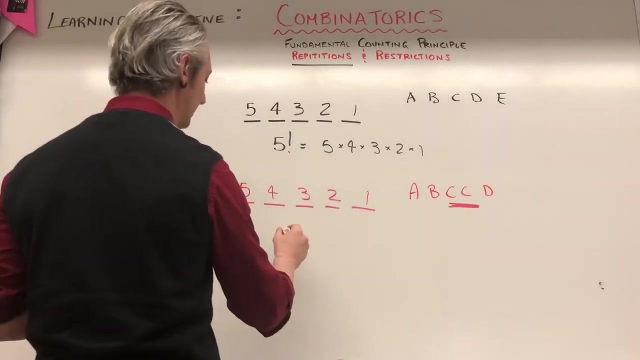 these are, these are. we can't tell the difference between this C and that C. okay, How many unique ways can we arrange those five letters? And in this case it's the same thing. it's going to be five times, four times, three times, two times one. However, at the end we need to divide by the amount of repeated objects: factorial. So in this case I have two repeated C's, So I this becomes five. factorial divided by two: factorial, And then that. 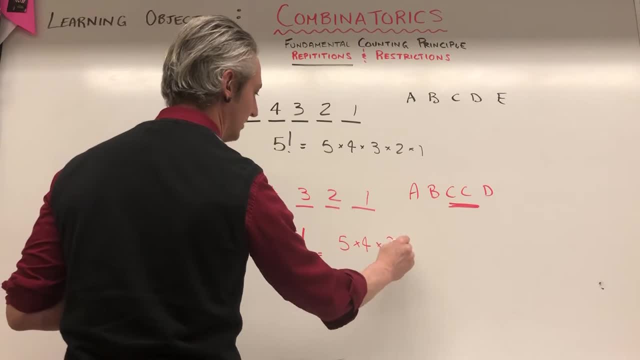 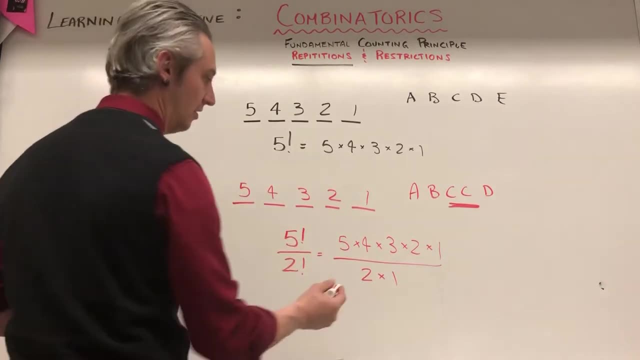 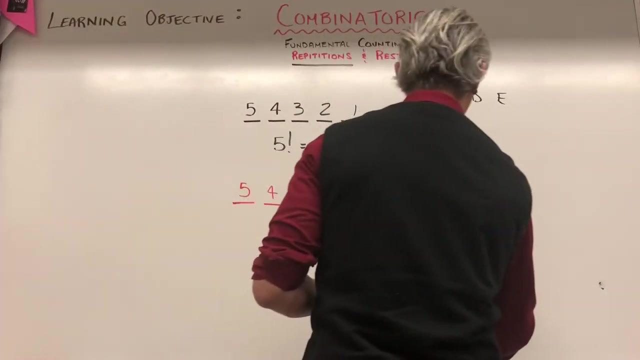 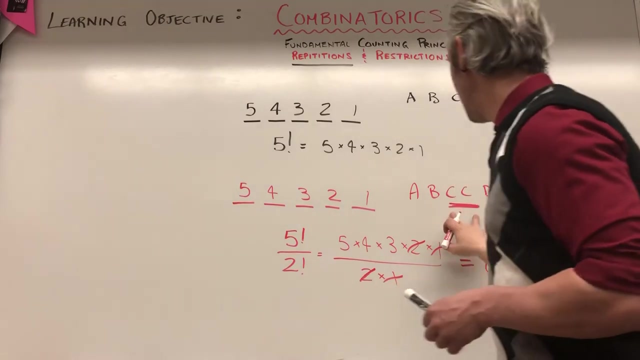 works out. So it works out to five times four times three times two times one, divided by two times one. And if I'm smart, I realized: oh, this cancels with that, that cancels with that, And then my answer is really just five times four times three, 60 ways, Versus up here it was five times four, which is 20,, 60,, 120. So as soon as I add two of the same object, I can only arrange them half as many unique ways. 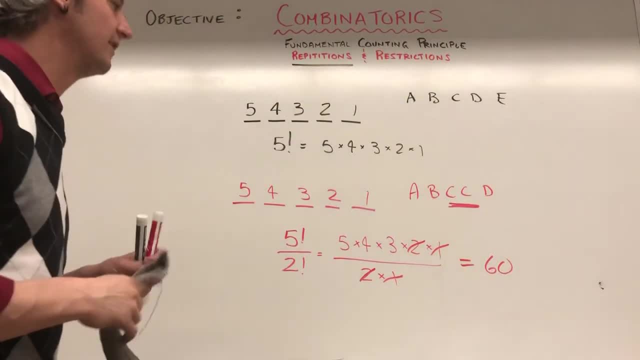 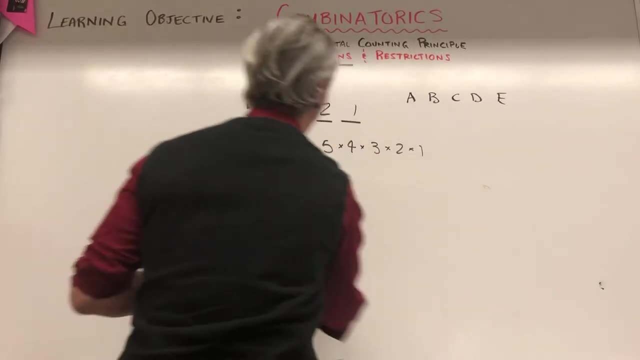 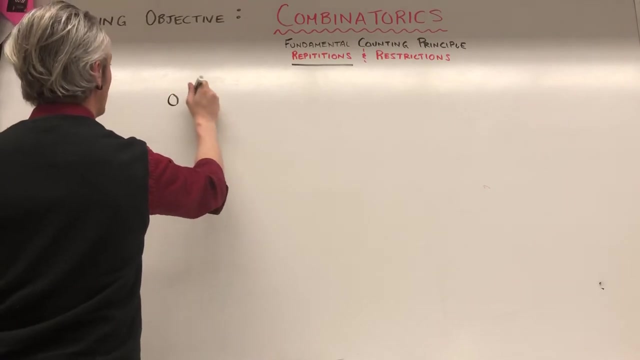 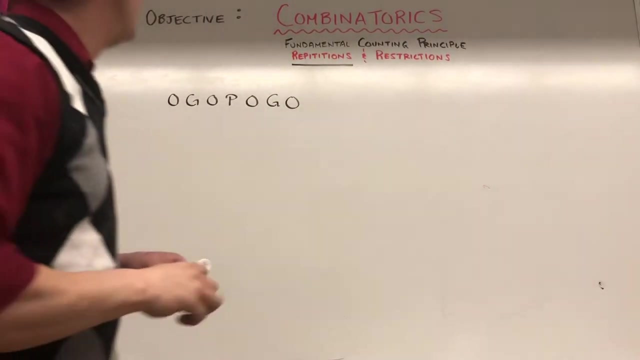 So let's do one slightly more difficult one, And then we're going to move on to restrictions, which is a little more involved, takes a little bit more thinking. I think this repetitions is really just knowing the formula. So what if I have the word olgopogo? I love mysticism, I love the idea of things being out there which we cannot explain with science. So let's talk about the olgopogo. 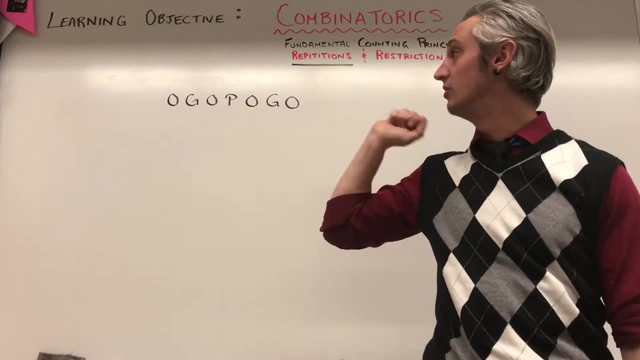 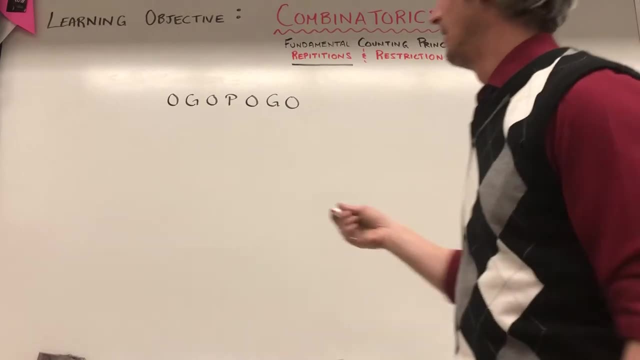 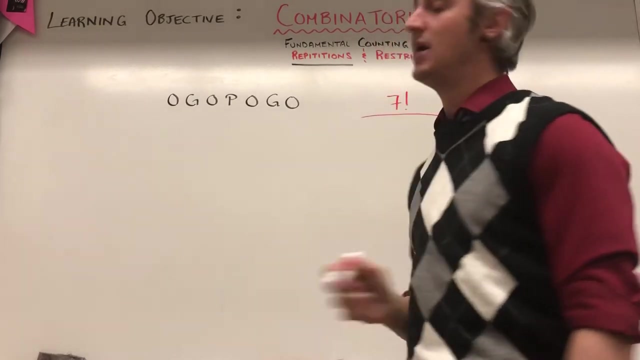 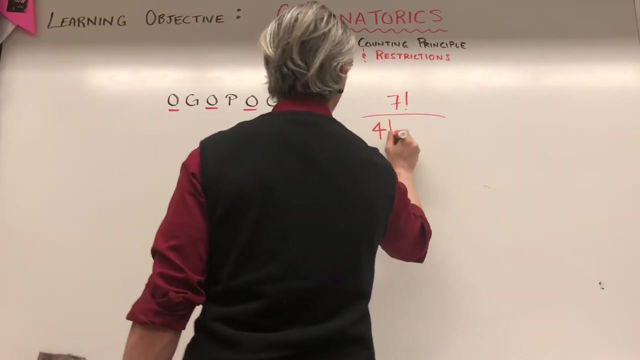 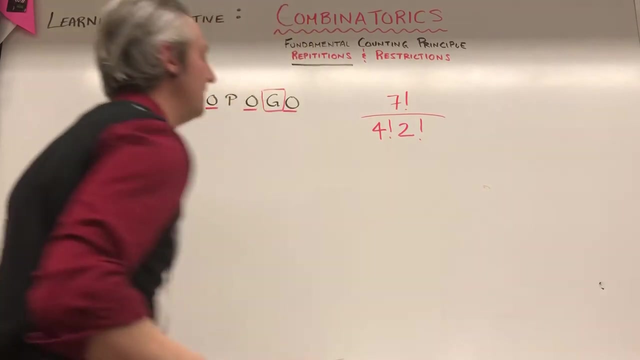 How many different ways? How many different ways can I arrange the letters in olgopogo to get unique combinations? Well, how many letters? One, two, three, four, five, six, seven. So that's going to be seven factorial. But then I have to divide it by my repeated object. So I have one, two, three, four O's, So I'm gonna have four factorial, And then I have one, two G's times two factorial. Okay, and that. 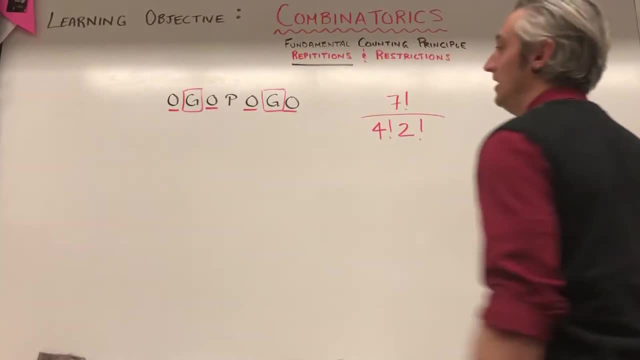 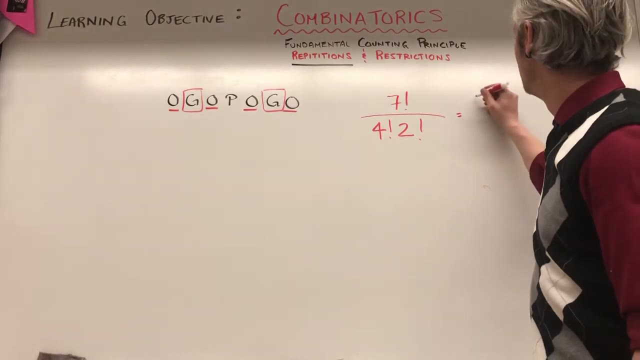 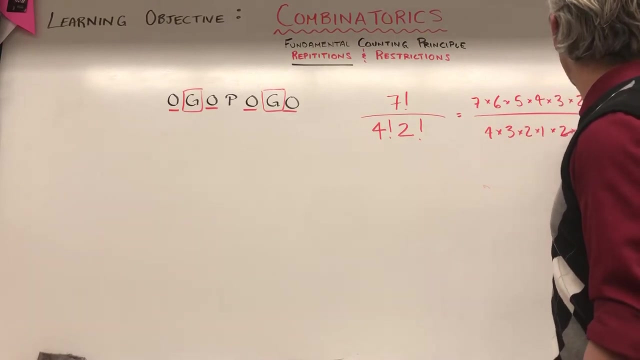 will give me the amount of combinations of those unique, unique combinations of these letters that I can get orders. And if I were to write this one out, I get seven times six times five times four times three times two times one, divided by four times three times two times one times two times one. This cancels with that Three, cancels with three or four, And then I get seven. 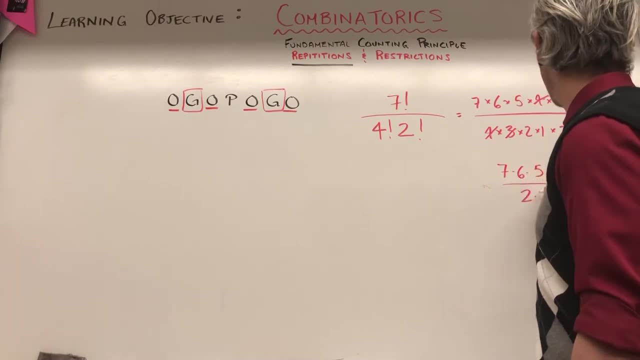 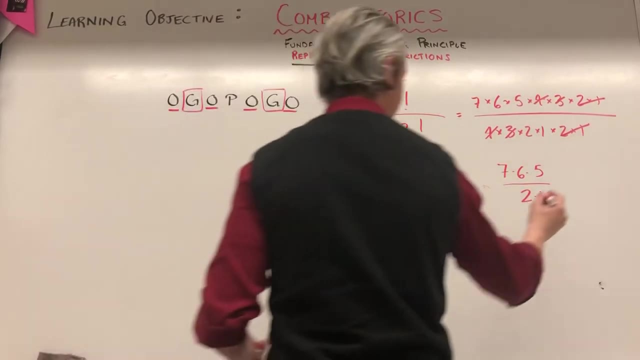 times 6, times 5, divided by 2, times 1.. And I do the math and I come up with: 7 times 6, times 5, divided by 2, I get 105 unique combinations of these letters Unique. 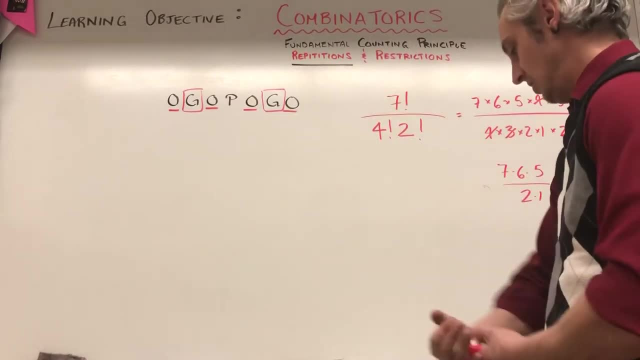 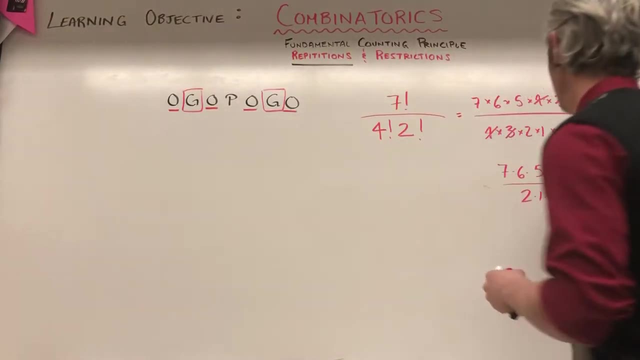 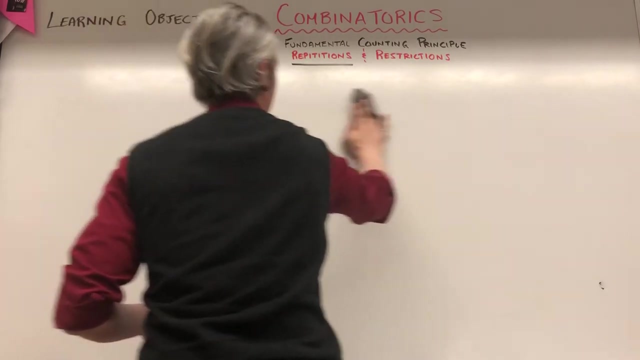 Okay, So that is repetitions. There's not much more to tell you. I think you'll be able to figure that out. Okay, So what happens now if we get restrictions? So what's under restriction? Let's go back to our 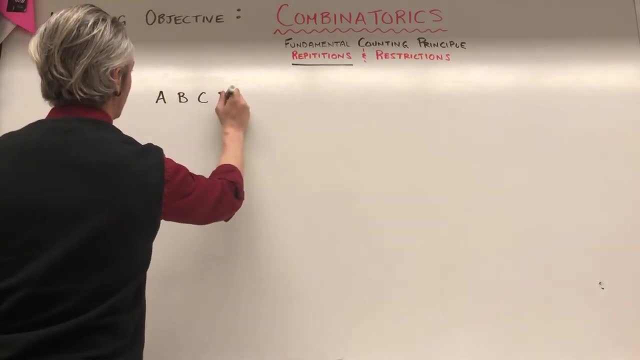 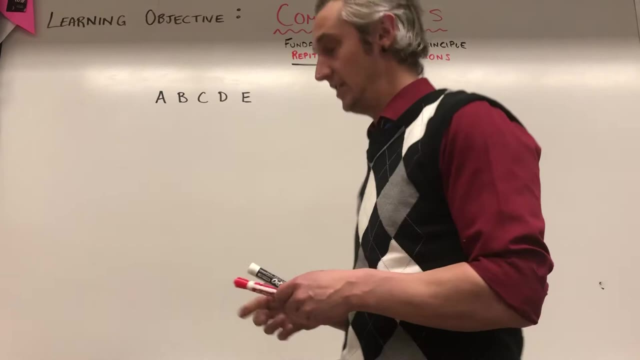 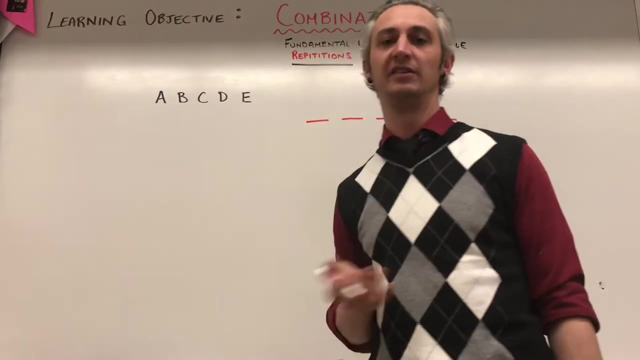 A, B, C, D, Okay, And restrictions, just they require us to start thinking a little bit Right. And it's always good to draw this stuff out. So if I said how many different ways can you arrange these letters, You'd say: 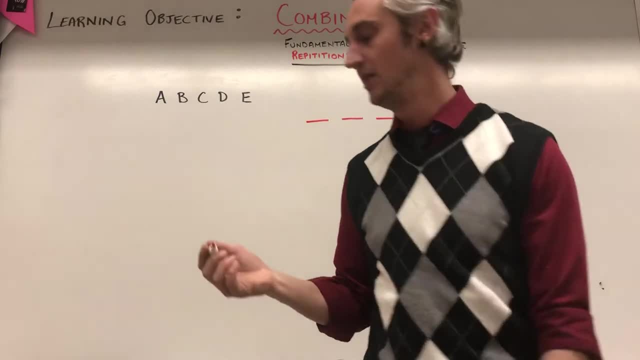 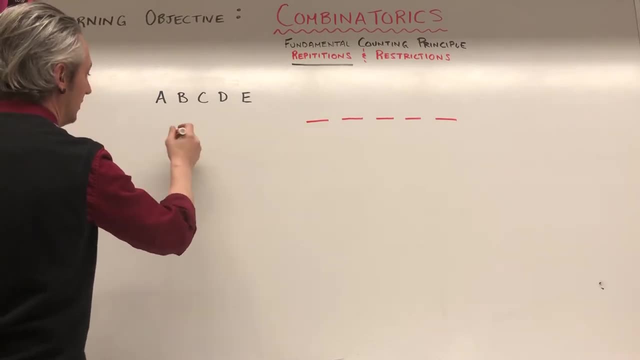 5 factorial. 1,, 2,, 3,, 4,, 5. 5 factorial. Now what if I said: how many ways can you arrange these letters so that C is always in the middle? Okay, So basically we're saying this is a restriction. 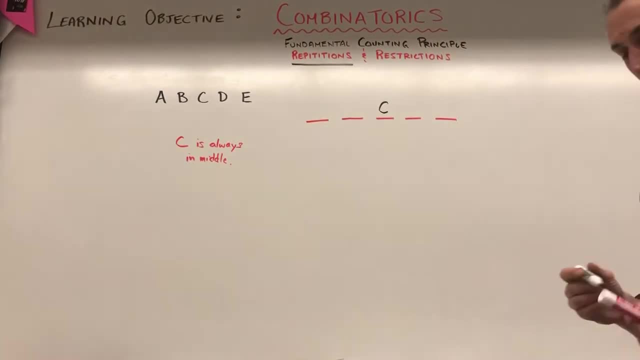 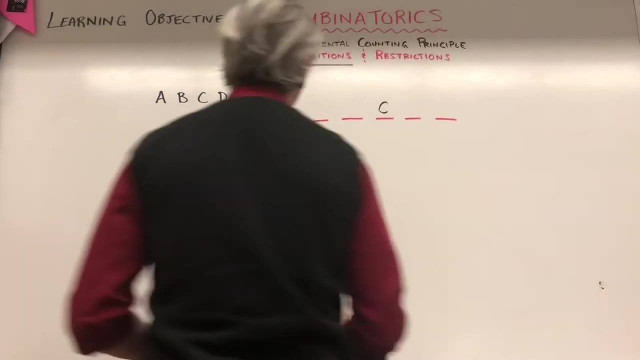 C is always right here. How many ways can you arrange these letters? Well now, if we can't really do factorial now because it's getting messed up by this, So what we do is we just have to start thinking about it. Well, how many choices. 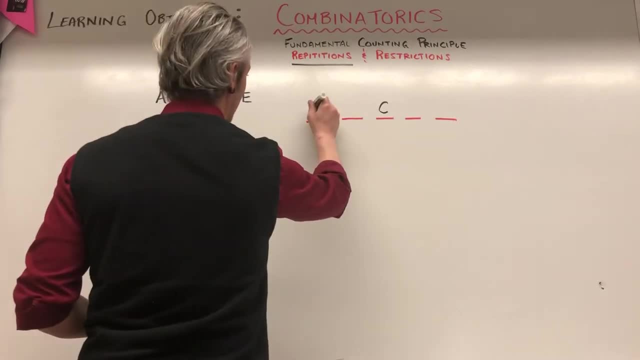 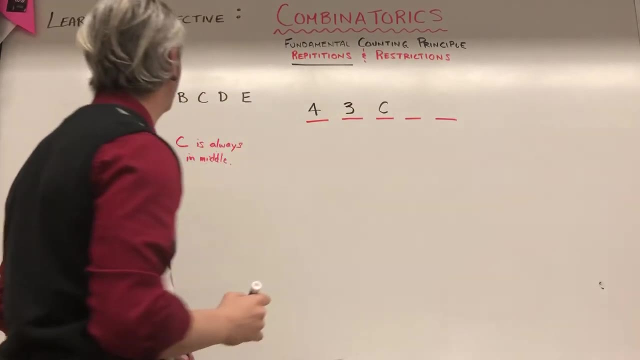 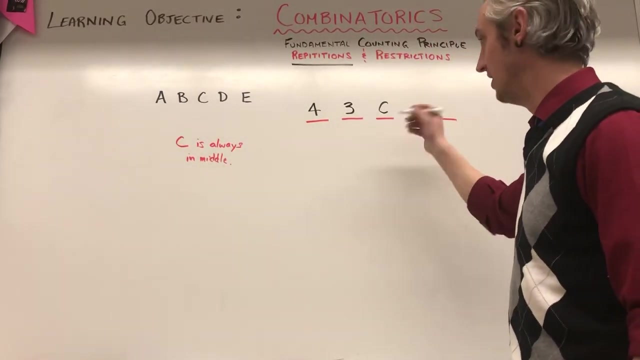 do I have for the first slot? 4. How many choices do I have for my second slot? 3. C, that's always. it's only one choice. so that's just a 1, or C. I can change that with 1.. It's 1.. 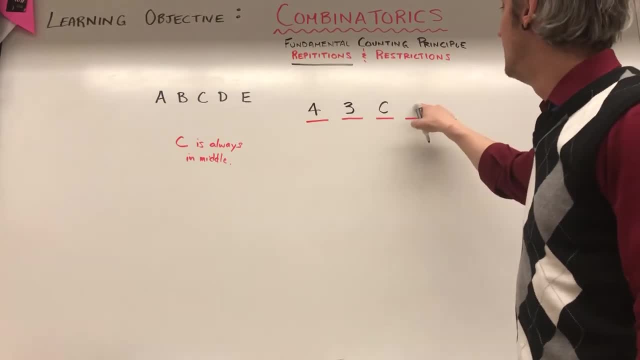 But I'm just going to leave the C there because 1's not going to change the math. So how many options do I have for this slot 2.. And how many options for this slot 1.. Now you might be asking: well, why do you always start on this? 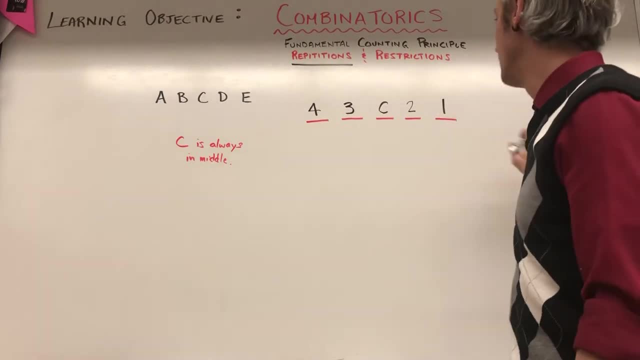 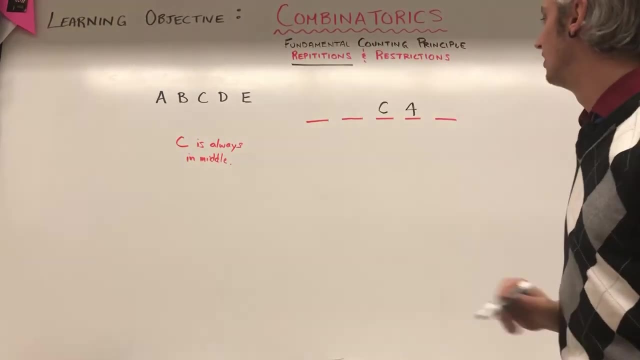 stage. Why do you always start on this on the left and move your way right? Well, I don't have to, Because if I'm multiplying all of these anyways, if I started on this chair, well, there's 4 choices for this chair. 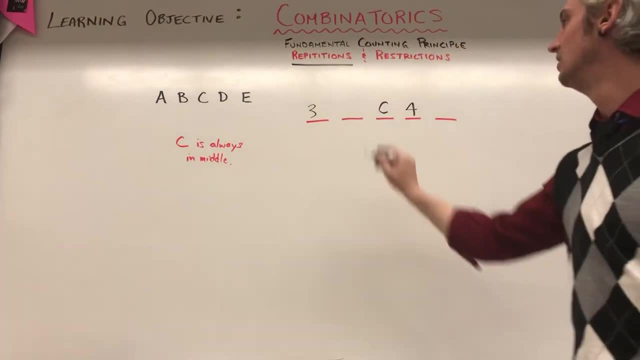 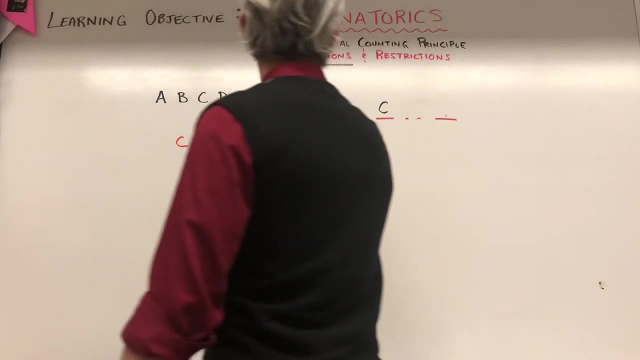 And then if I came over here next, there's 3 choices there, 2 choices here, 1 choice there, And if I multiplied it out it's the same as if I went 4,, 3,, 2,, 1.. And so I get. 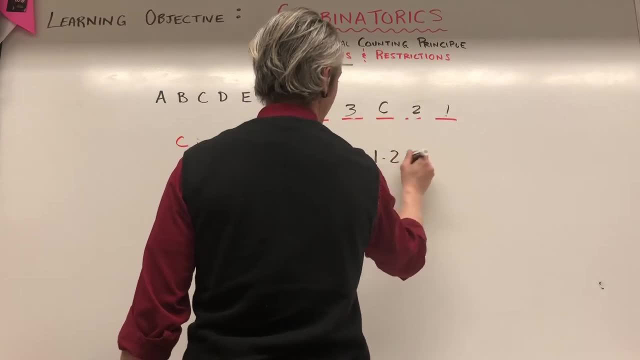 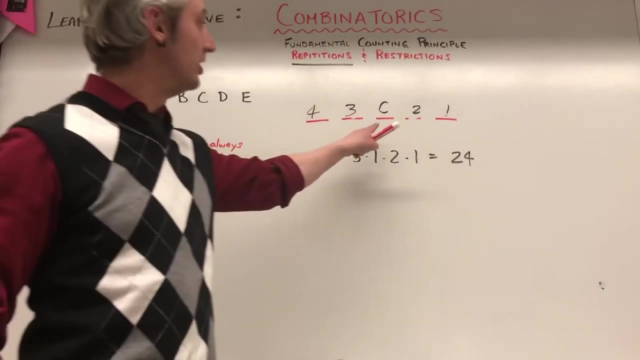 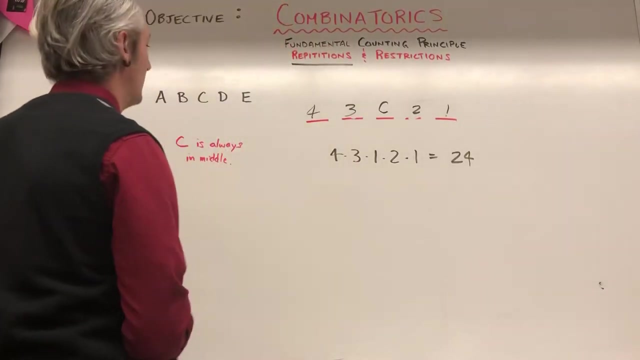 4 times 3 times 1 times 2 times 1, 12, 24. 24. Different ways. when I have the restriction that C is in the middle, Okay, What if I had a different restriction? What if I had? 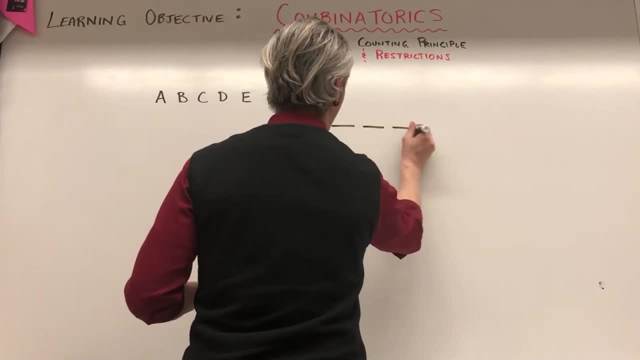 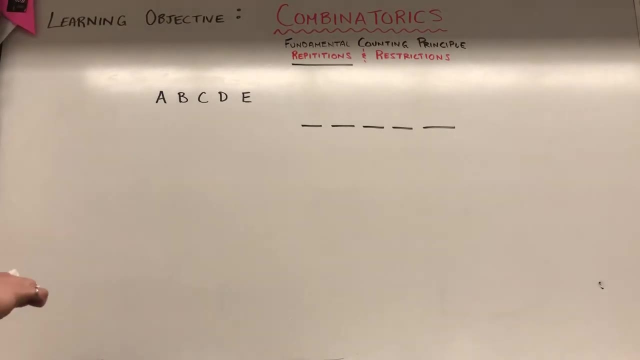 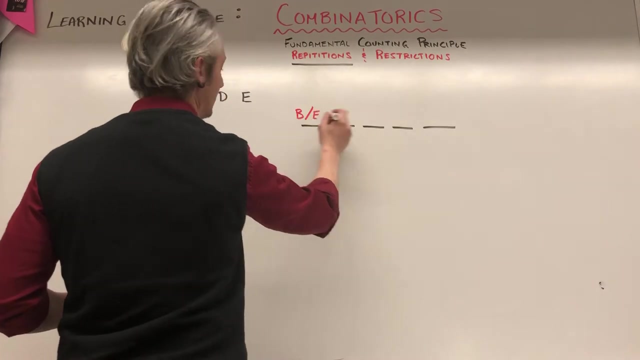 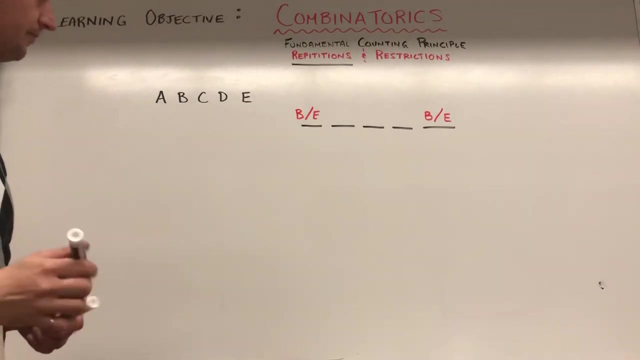 the restriction that B and E must be on the ends. So this is either B or E, and then this is either B or E. Well, how would that one be done? Well, what are your choices for the ends here? Let's say, I start on this one. 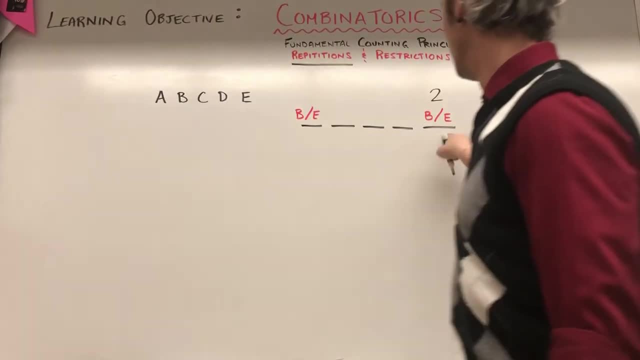 Well, I have 2 choices- B or E- And if I have 2 choices here, by selecting 1, I'm left with 1 choice on the other end And I could have done it the other way. I could have done 2 choices here. 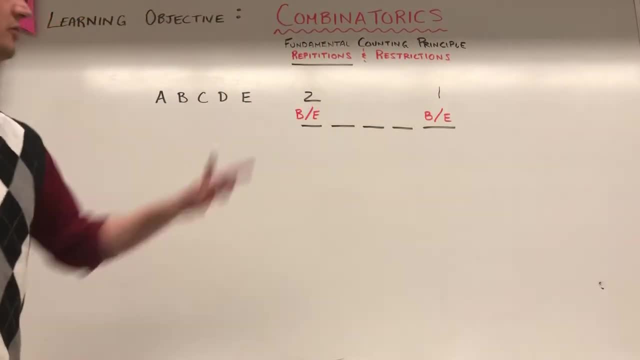 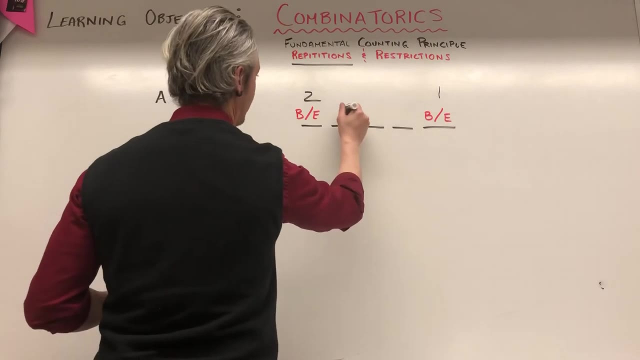 leaves me with 1 choice here. So there, we've got 2 out of the 5.. And then the rest. it doesn't matter where I start. I have 3 choices here. now. I have 2 choices here and I have 1 choice here. 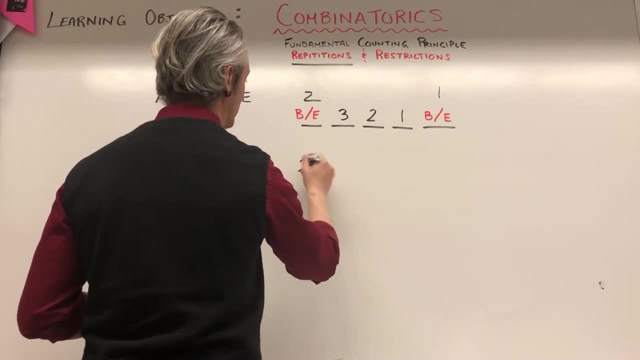 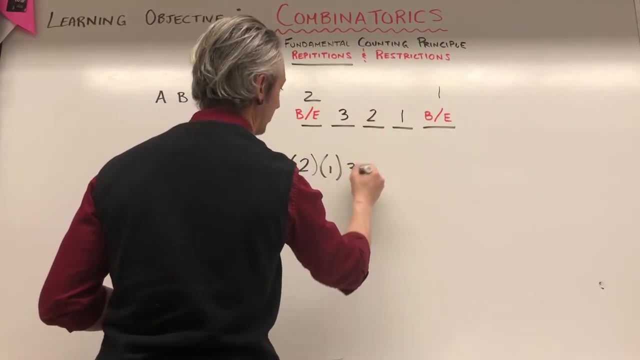 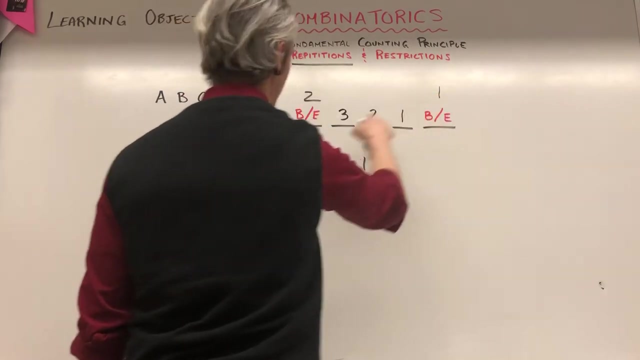 And therefore my answer is 2 times 1 times 3, times 2 times 1 or times 3 factorial, And if I do that I get 2, 2 times 1, and it doesn't matter which way I do the multiplication. 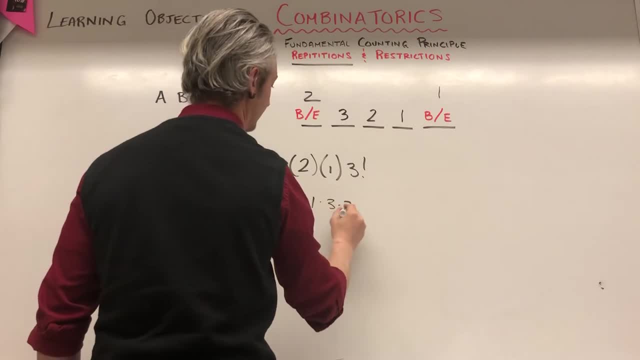 I'm just trying to show you: 2 times 1 times 3 times 2 times 1, 2 times 3 is 6, times 2 is 12.. 12 ways when I have an additional restriction which makes sense. 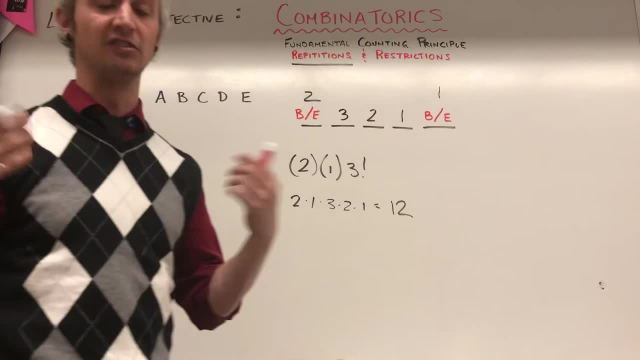 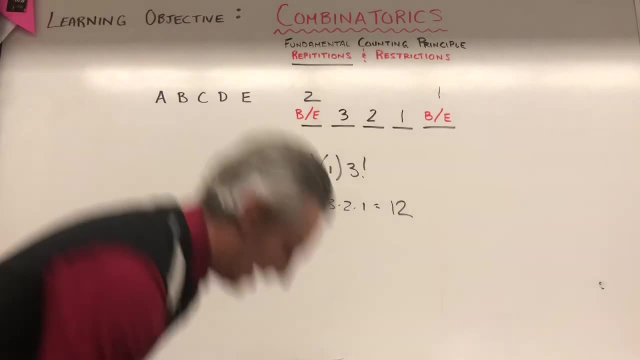 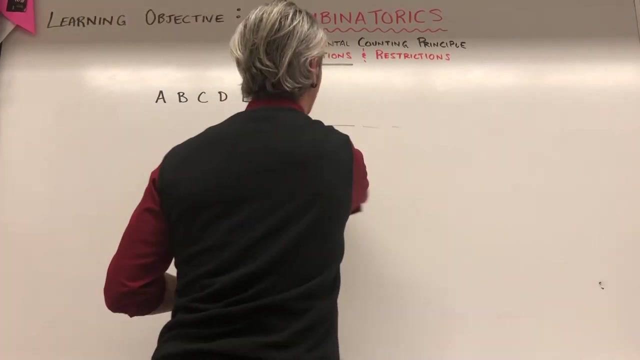 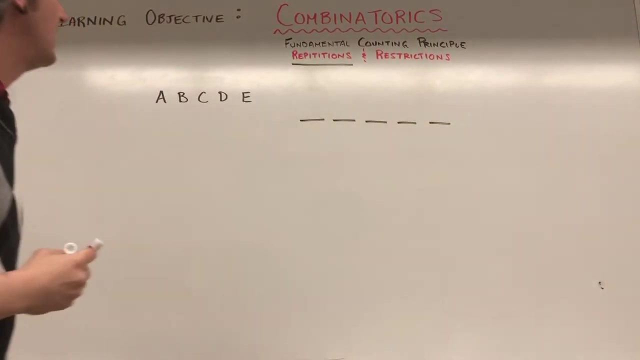 I should have less ways of ordering them when I have more restrictions. The more restrictions, the less amount of ways I can achieve something. Ah, okay, Okay. What if I said: how many ways can you arrange these letters if D and E? 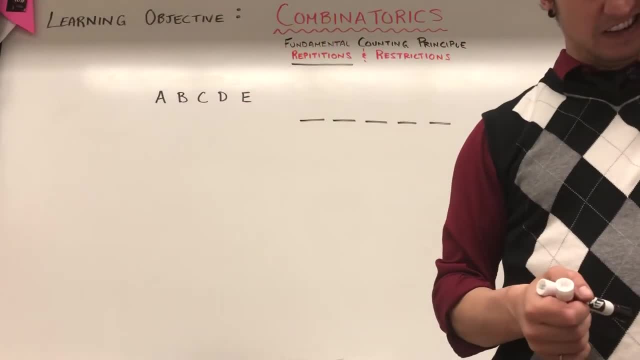 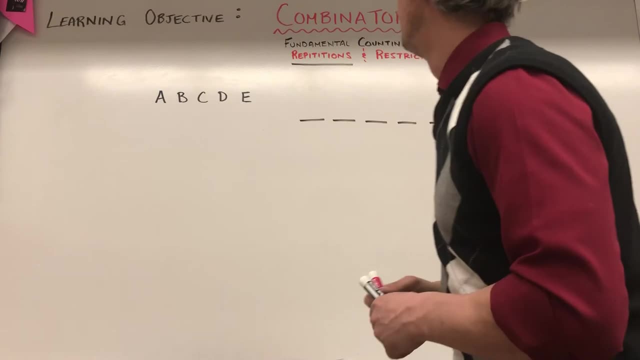 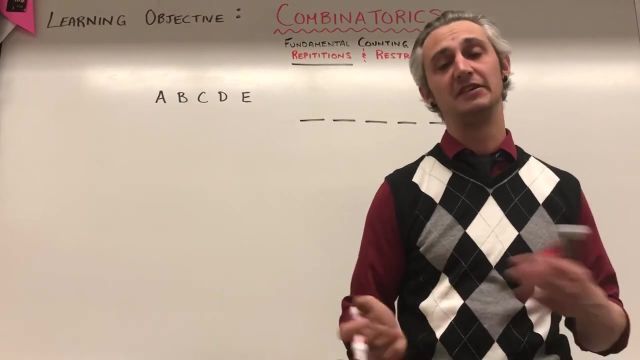 have to always be beside each other. Okay, D and E now have to always be beside each other. So what happens in this case? Now, this is where it starts to. you start to kind of learn how different scenarios play out. And in this scenario, 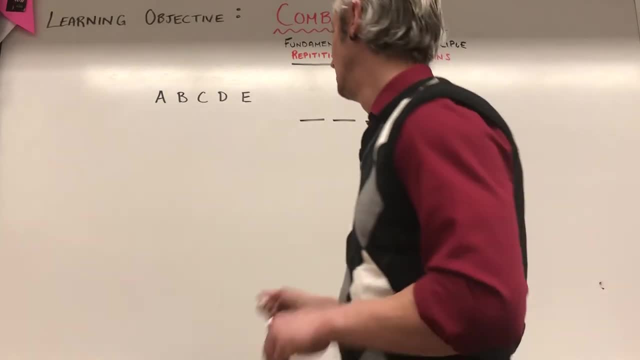 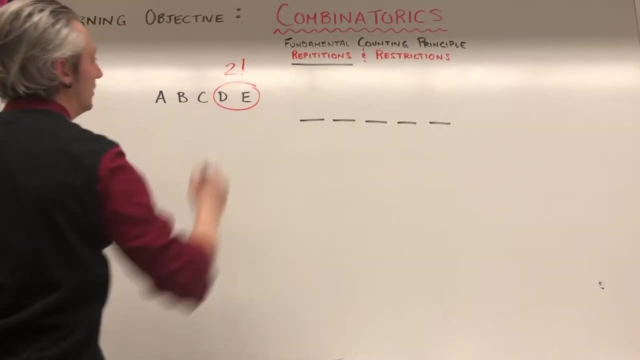 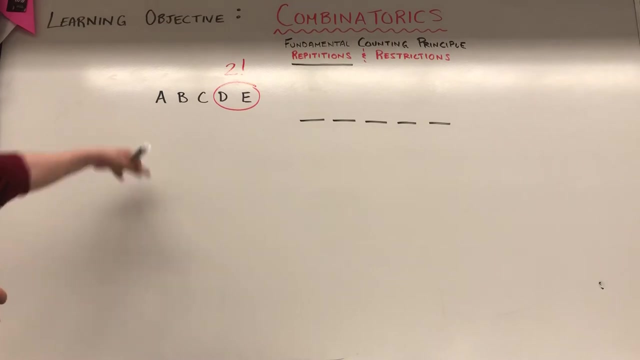 when you have a restriction where two things have to be together all the time, well then, essentially those two things become one object with two factorial possibilities, And then then you can just treat this as so. if you're treating this as an object, 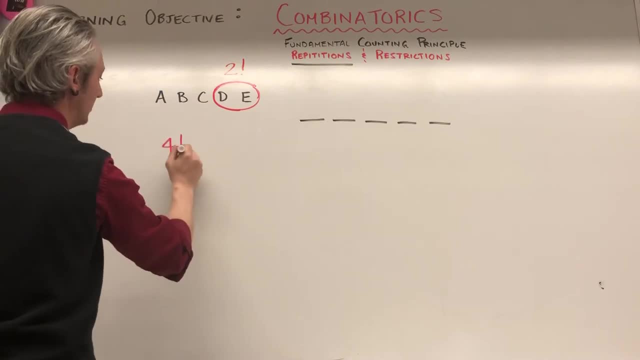 then your solution is 4, factorial, because I have 1,, 2,, 3,, 4 objects. but then I have two ways of ordering the D and the E Right. So pretty much one option is A, B, C, D, E. 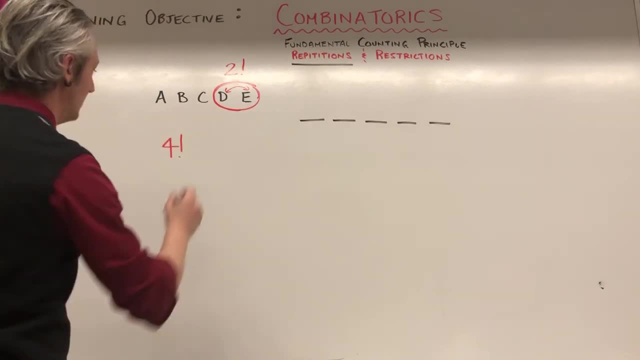 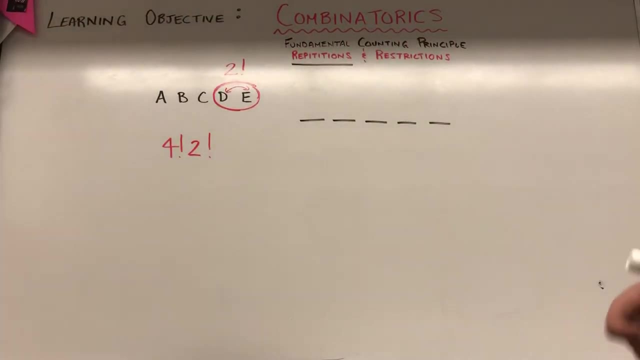 and then another unique one would be A, B, C, E, D, So 4 factorial times 2 factorial. That's what happens when you have objects that need to be beside each other. If I said that, the C and the D and the E. 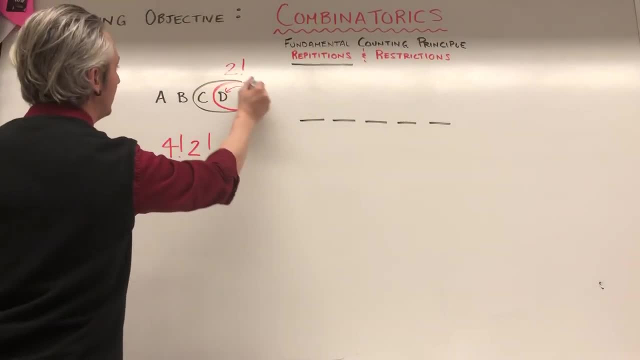 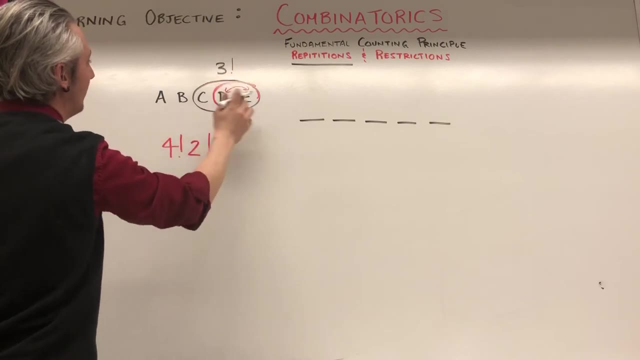 had to always wind up grouped together in one group where the C and the D and the E are beside each other. well, now, there's three factorial ways of ordering these, but then if these are going to be treated as one object, then I have 1,, 2,, 3- factorial. 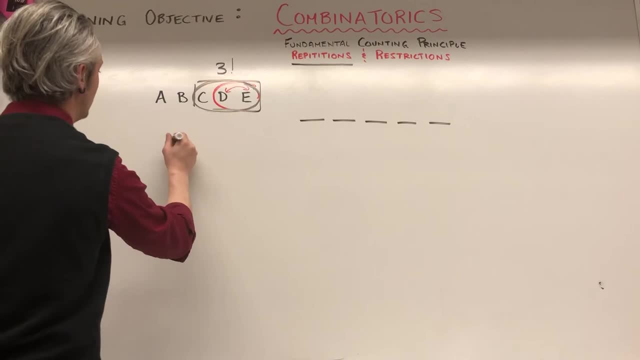 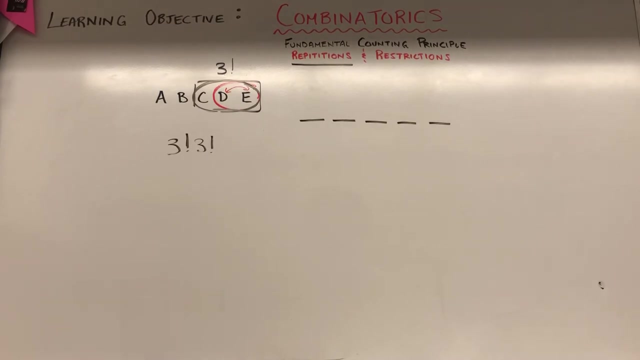 so it's 3 factorial times 3 factorial Right, Because I'm ordering these objects, but then I'm ordering these ones inside. Hi Rachel, How did you find some point Just here? I don't have all, just everybody is supposed to have a point. 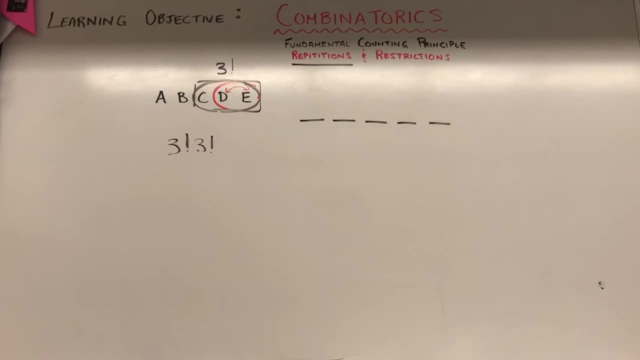 Okay, Is everybody supposed to sign it? Yep, It goes back to each other. Okay, Thank you, Appreciate it. Thank you for hooking up for me. Thank you, She said not even just the custodians, it's everybody. 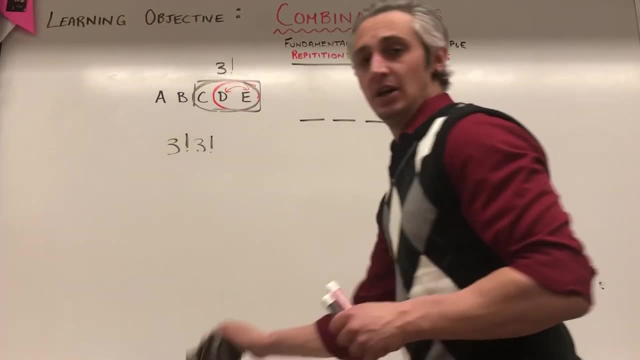 Okay, I should read my e-mail, shouldn't I? Yeah, Okay, Thanks, Rachel, You're welcome. Okay, So, and then there's one in the textbook. Actually, I'm not even going to read that one just yet. 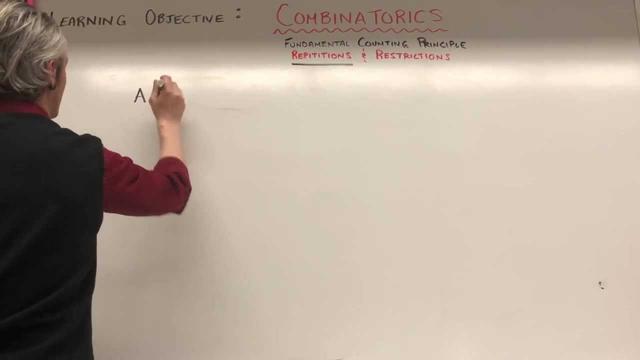 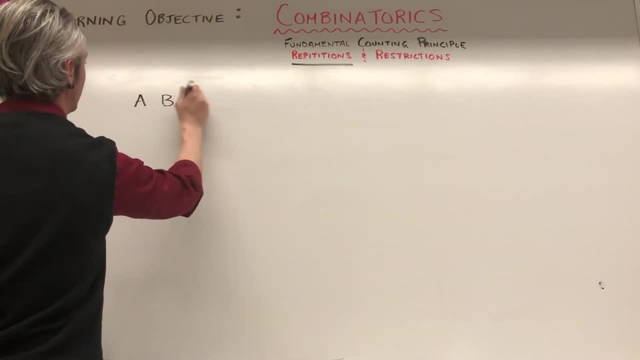 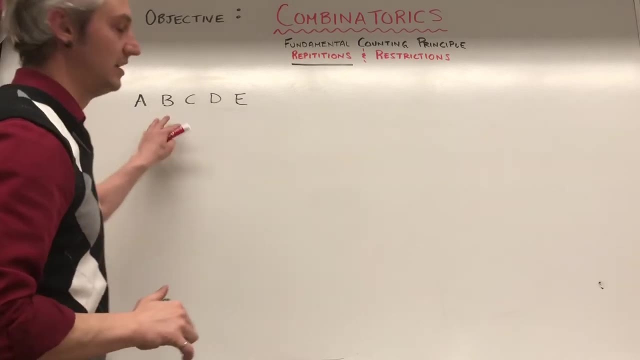 Great question. So what if I had a, b, c and d and e? This is a thinking problem And I said: okay, a and b can never be beside each other. How many ways can you sort these out? 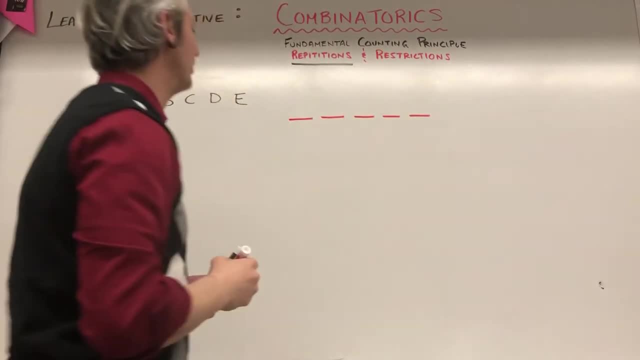 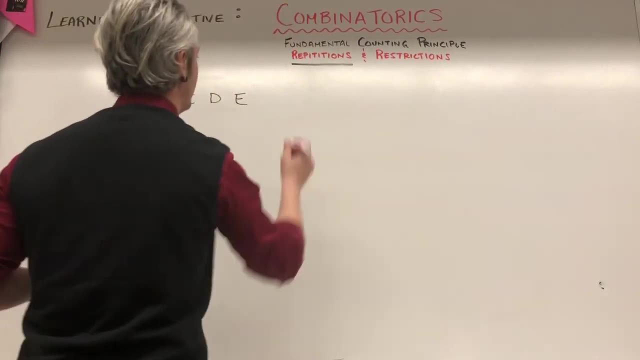 In this case we have to figure out all the different ways. that a and b can never be beside each other. Okay, So I can have a space b space space where a and b are not beside each other. Okay, So you can interchange them. 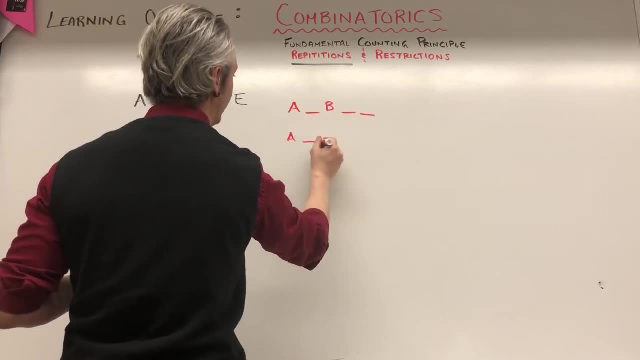 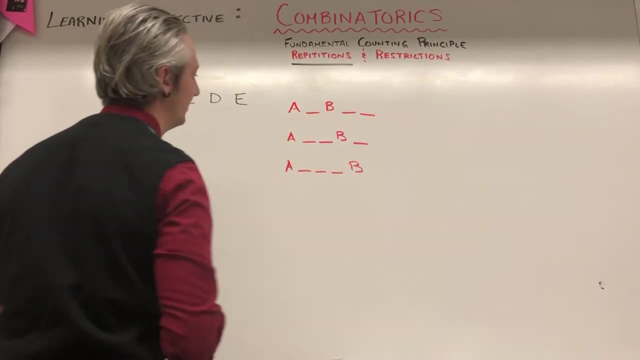 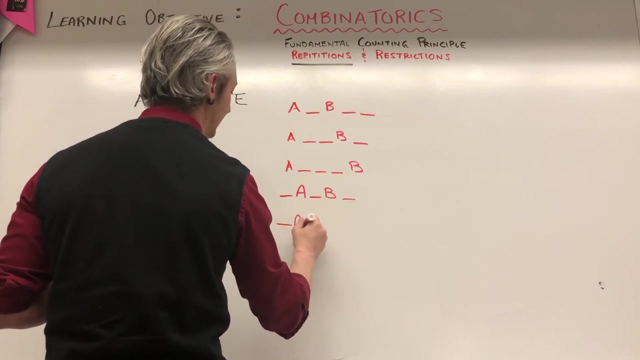 I'm just trying to figure out all the ways I can have a space, space, b, space where a and b can interchange. I can have a space space, space b on the ends And then I can have space, a space, b space. I can have space a space, space b. 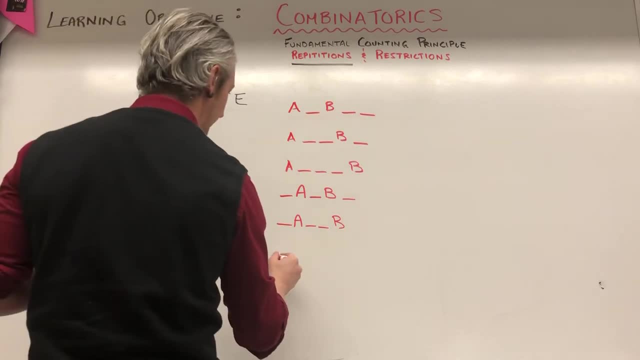 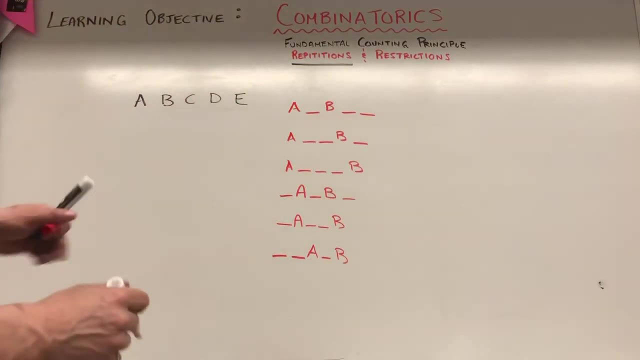 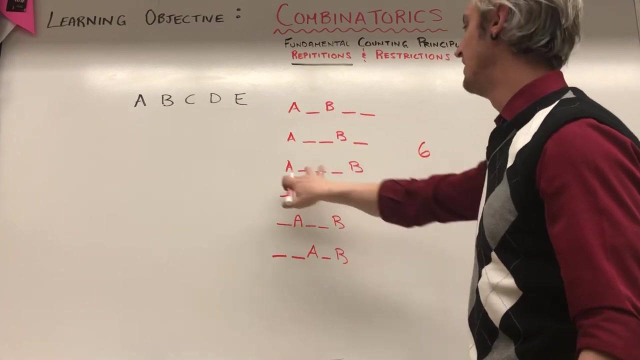 And then I can have space space, a space b, Okay, And then I can have a space space, a space b, And, assuming that I can interchange A and B together, there's six different ways. so there's six ways of not having A and B together, and then I have to multiply. 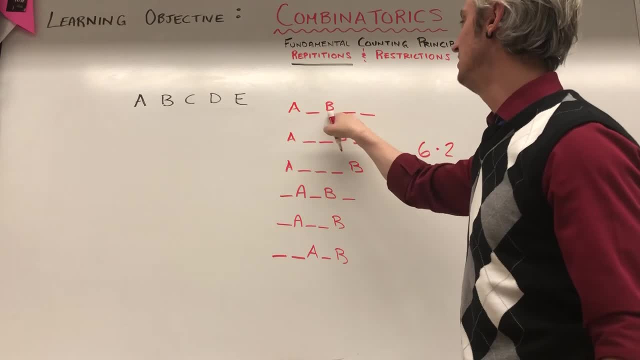 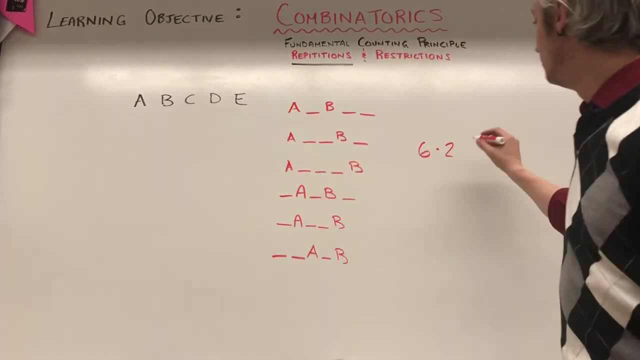 that by two, because A and B are interchangeable. So A and B is different from B and A with the same thing. so six times two, That's all the ways I can order the A and the B, but then I have to multiply it by well, how can I order the? 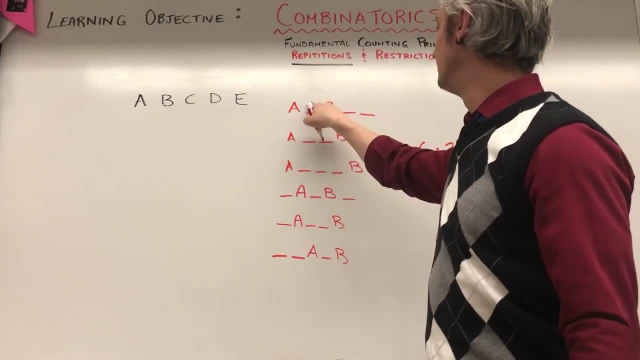 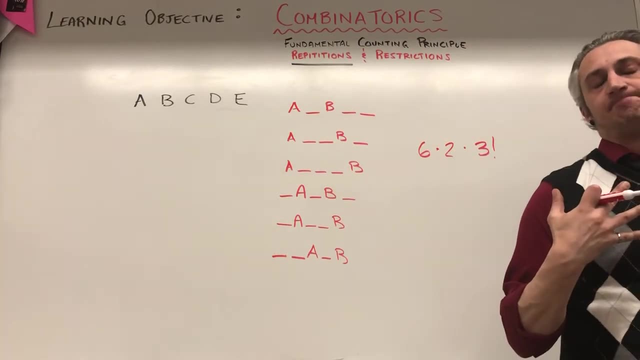 rest. Well, it's going to be. there's three options for this slot, two options, one option. so then it's times three: factorial. Probably confusing first time looking at it, that's okay. I remember when I did this in math it was. 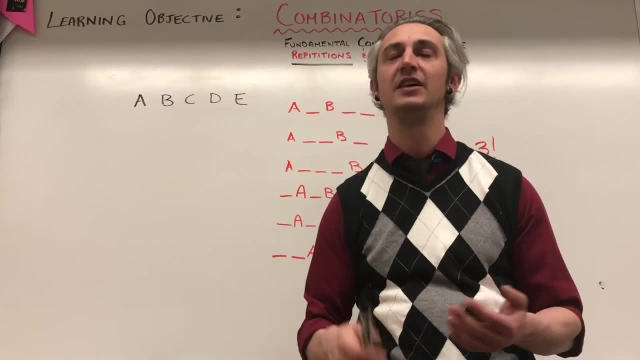 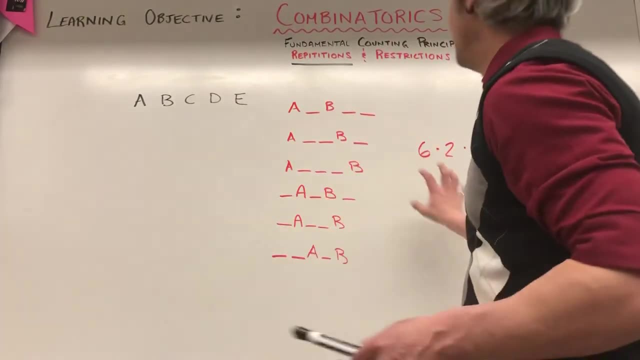 tough. it was tough, it was hard to learn, but you got if you do more problems. this is really a unit where you have to do a ton of practice problems to really get a feel for all the different scenarios. but that's how you do. 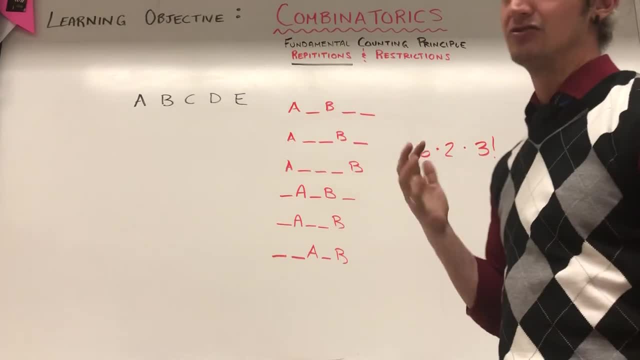 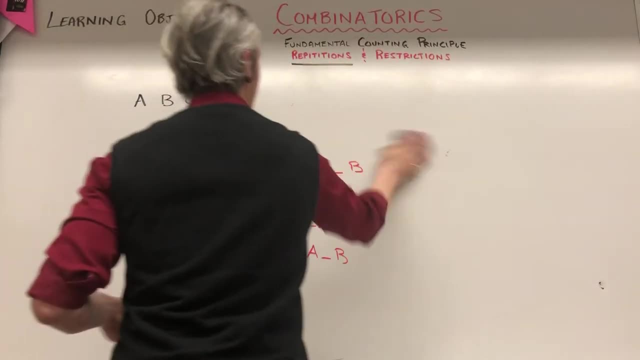 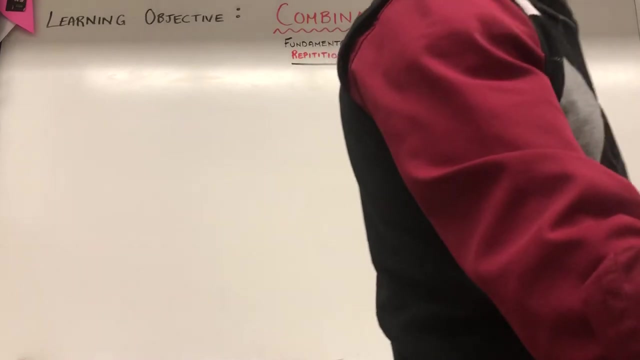 something when they have a restriction, where you're separating things and draw things out, write it out, work it through, But let's just do a textbook problem together and then I will send you off. okay, Let's see here So and how. 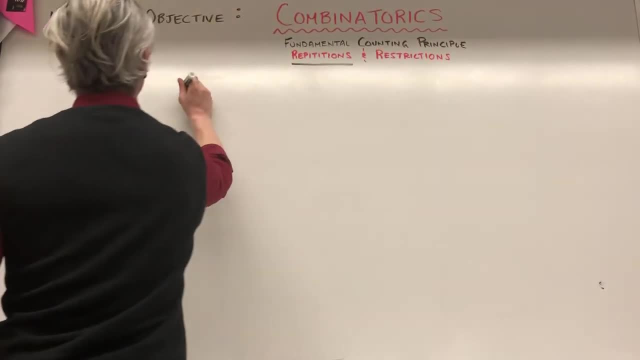 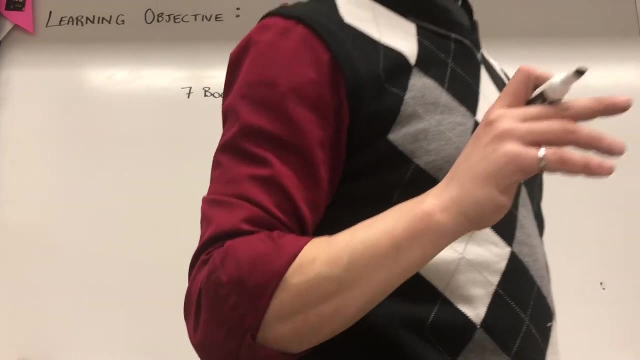 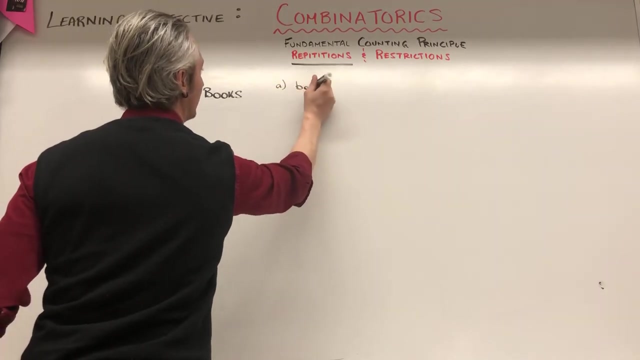 many ways can seven books be arranged on a shelf? I have seven books and I'm assuming all the books are unique. okay, How many ways can I arrange the books on a shelf if all the books are different? Okay, Books are different. There's no repeats, is what they're telling us? Books. 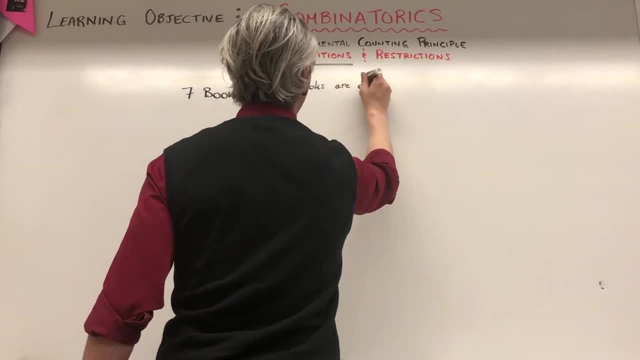 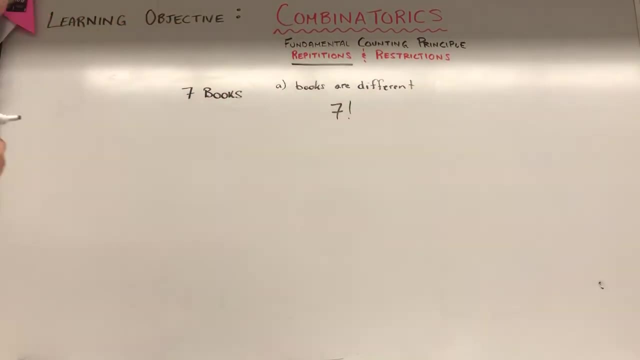 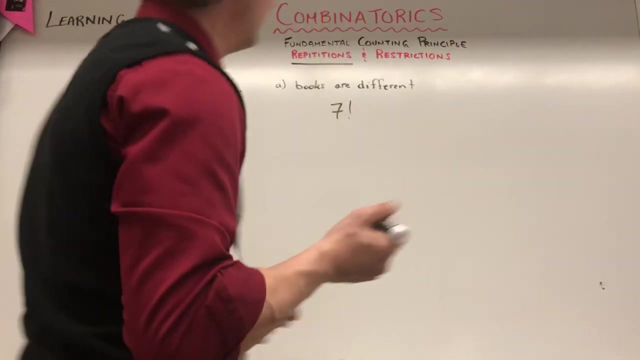 are different. So hopefully you've already yelled out the answer to me, and that answer would be seven factorial Seven books. there's seven factorial different ways. That first slot has seven options. That second slot has six options. Third slot: right, Because the order matters. So what happens if two of 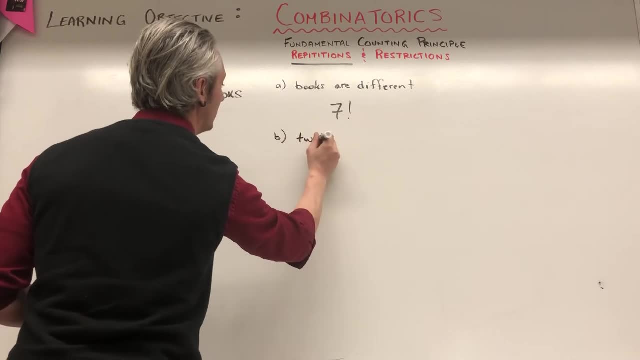 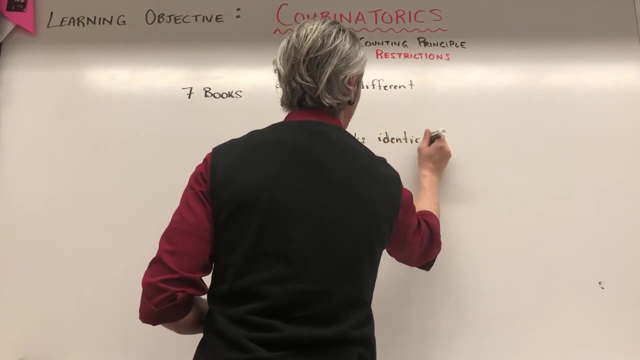 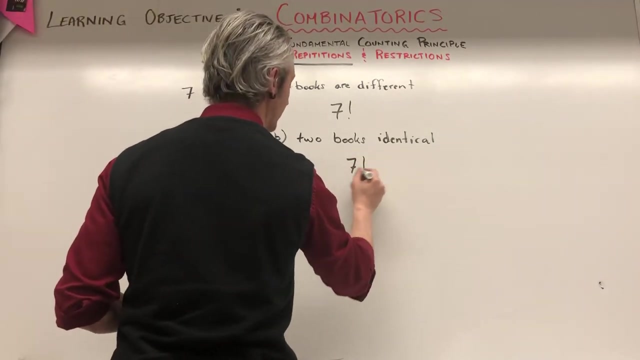 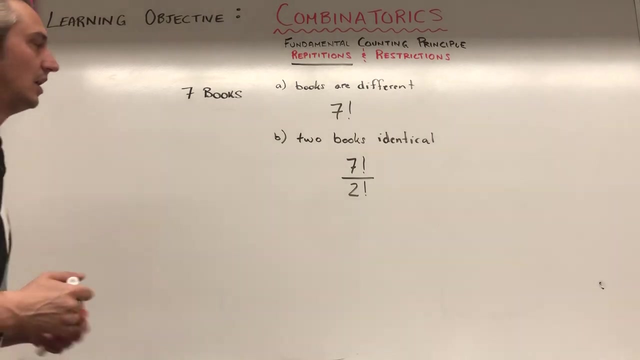 the books are identical. Two books are identical is another way of saying. I have two repeats. So in this case, if two books are identical, it's seven factorial divided by two factorial- my repeats. I have two repeats, two factorial on the bottom, I'm not. 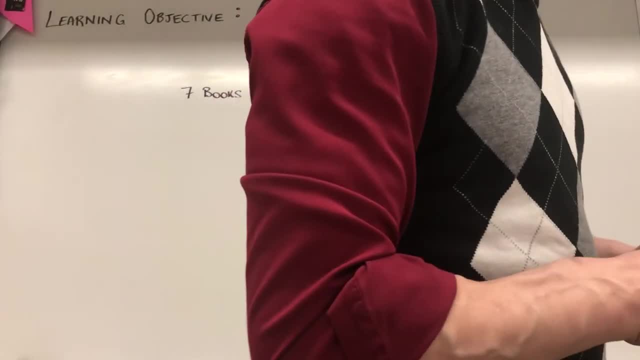 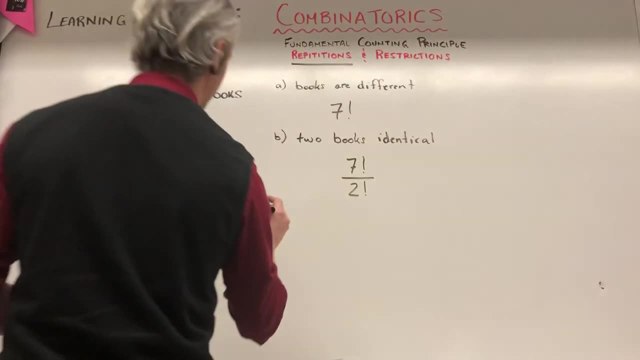 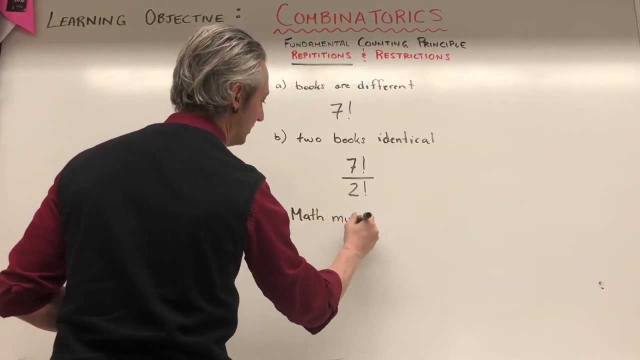 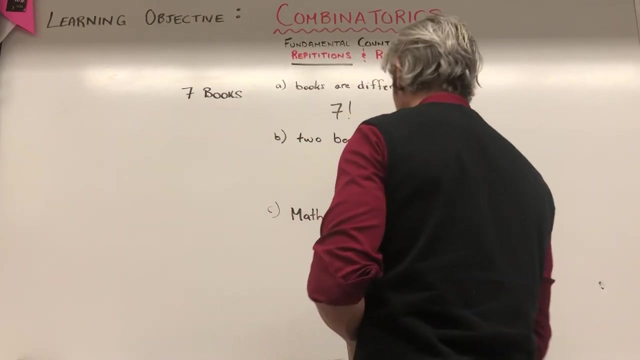 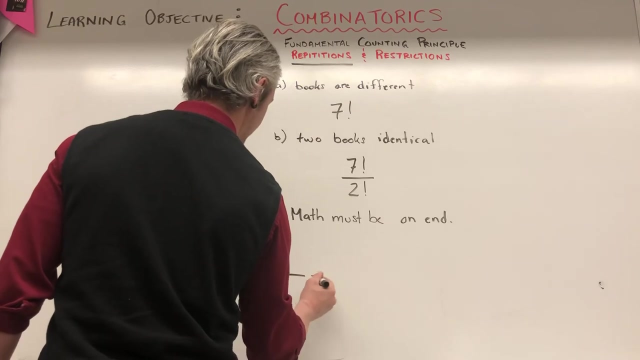 gonna solve an answer. You can do that on your calculator. See, the books are all different. The books are all different and the mathematics book must be on an end. So the books are still different. Math must be on an end. Okay, On an end. So that means 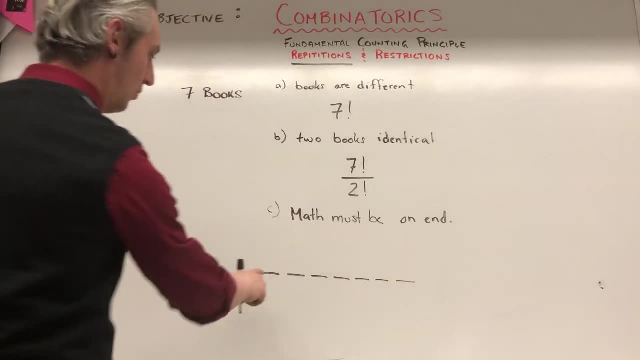 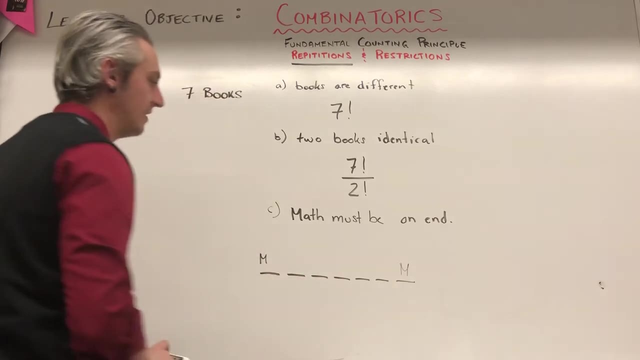 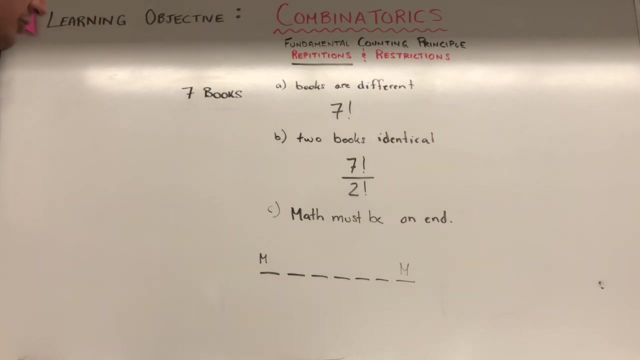 uh, uh, uh. one, two, three, four, five, six, seven. That means that I can have math either here or here. Okay, I have two options for the math book And then. so there's two options for the math book. Either that's my first. 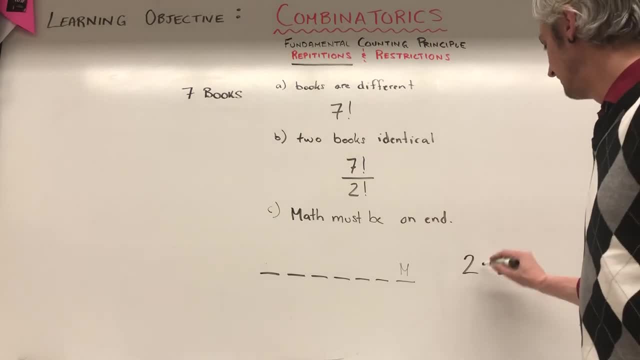 scenario, and this is my second scenario And then just like in the last, so this is kind of like the one where we did with uh. A and B being different places- They're more than a space away. Then the rest of the Latin book six. I have six different ways, So I'm 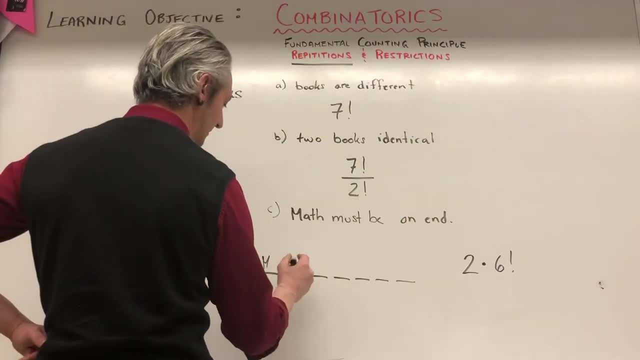 gonna have one option where I have my math book here and then I have six factorial. But then I have a second option- so that's why I multiply it by two- where I'm gonna have six factorial here and then my math book is gonna be on this end. So then I'm